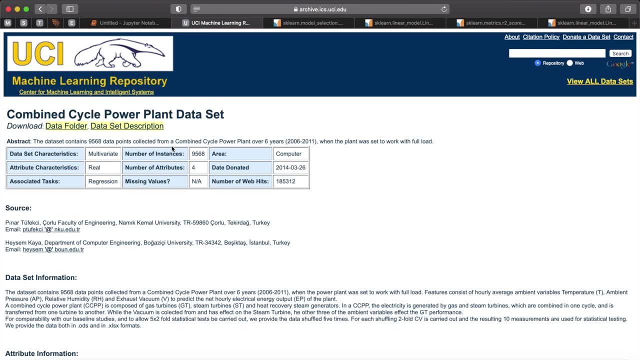 a combined cycle power plant over a period of six years, that is, from 2006 to 2011.. There are no missing values in the data. Number of attributes that we have in this data are four. Now let us see what is missing. 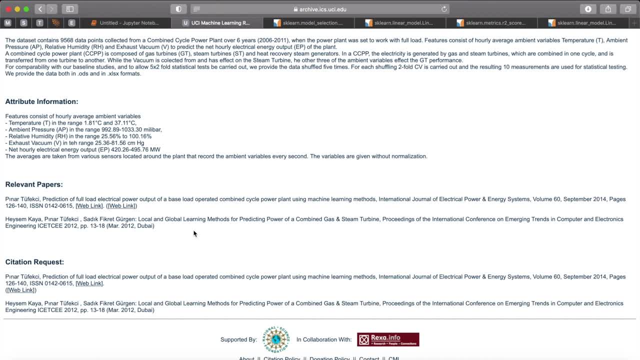 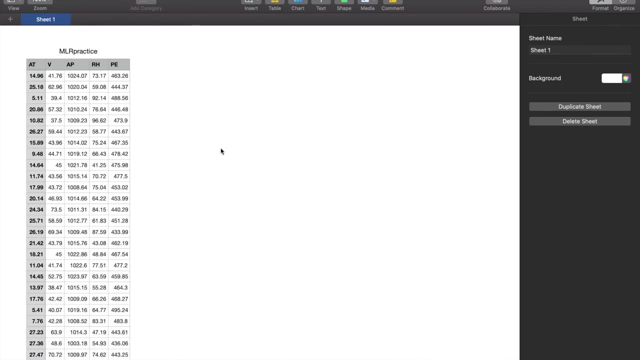 So let us see what are the columns that we have in this data set. So, as I have mentioned, I have already downloaded this data, The let me let me first show you how this data set look like. This is the data set that I have downloaded. it has five columns: ATV, AP, RH and PE. the 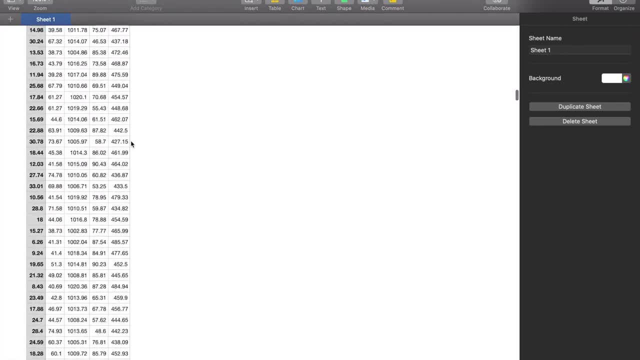 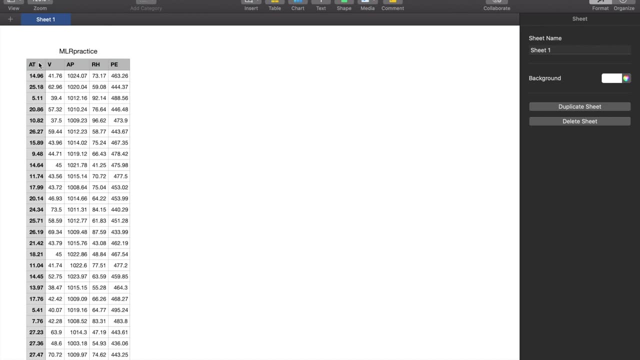 date. The rows that we have have Our, our boxes. One letter. We have two rows, So let us first look at this piece. So I have approximately 10,000. now let's see what these the name of the columns represents. 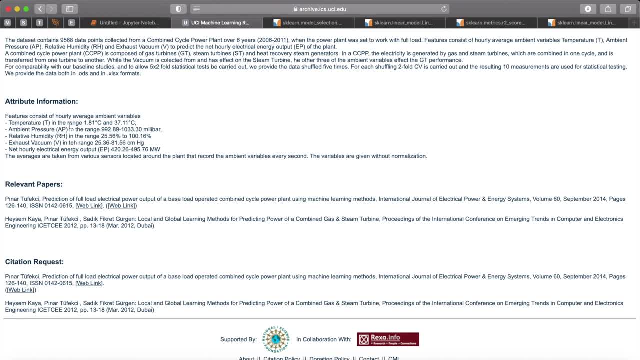 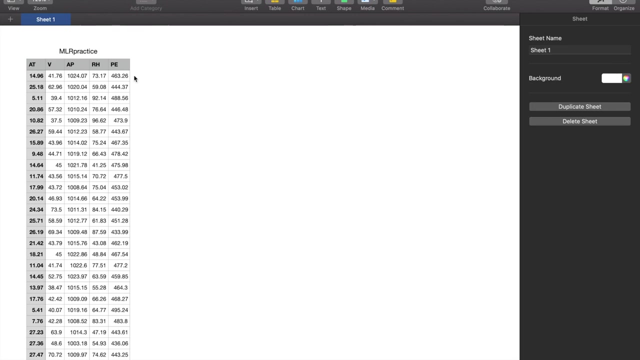 so 80 here refers to temperature, which is in the range from 1.8. 1 degree Celsius to 36, 37 point 11 degree Celsius. V is exhaust vacuum, AP is ambient pressure, RH would be a relative humidity and the last one that would be: 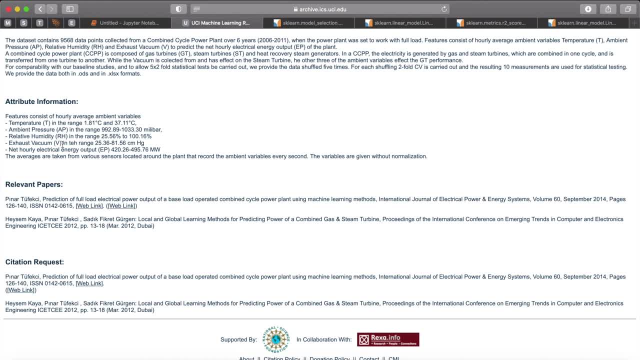 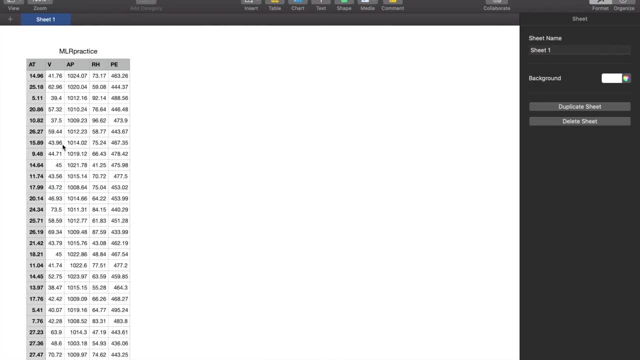 our dependent variable, that is PE, which is nothing but electric net early electrical energy output. so these are the data points that we have in our data set. so once you download this data, you and once you identify which are your independent and you and once you identify which are your independent and. 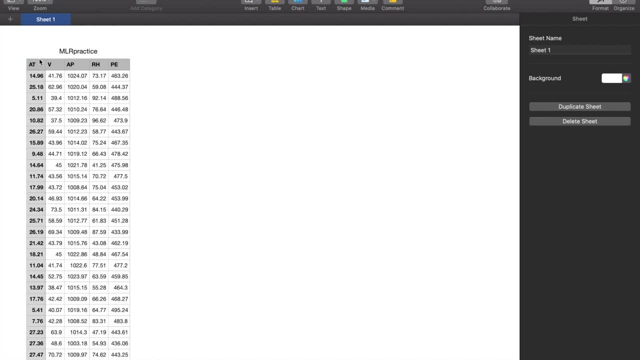 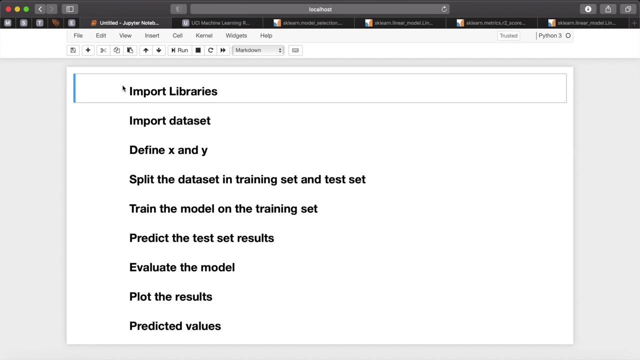 independent variables and dependent variables. so in this case, our independent variables are the first four columns, whereas our dependent variable is the last column, that is, PE. we will start now. we will now start building our model. here is our Jupiter notebook. I have already added the steps that we 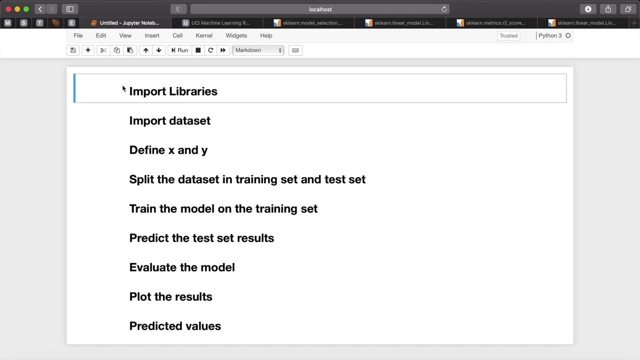 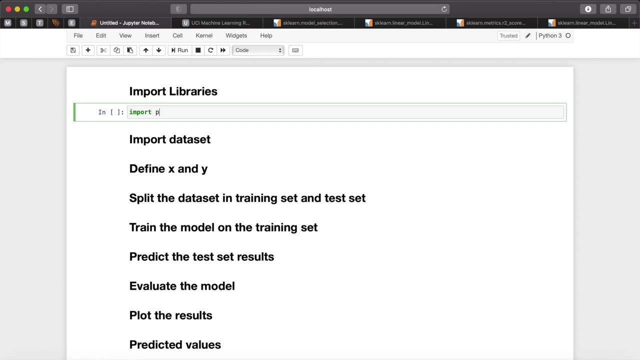 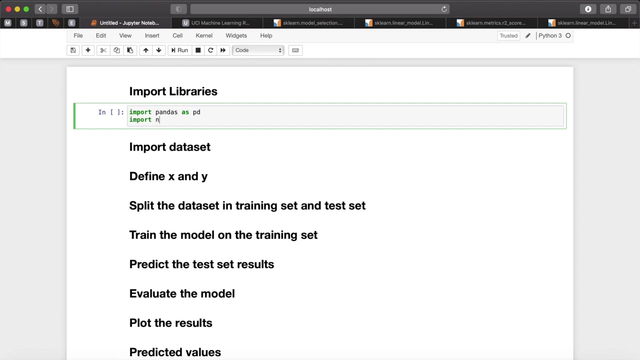 need to follow for our MLR model in the notebook. now let's start with building our model. the first and foremost step for us would be to import libraries. so let's start with importing the libraries and the data set. first library that we need to import as pandas, let us also import numpy as of now. 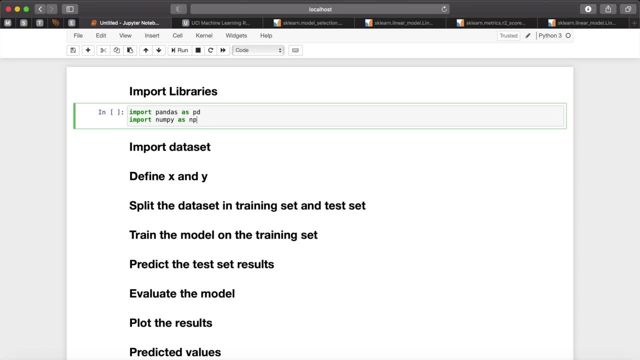 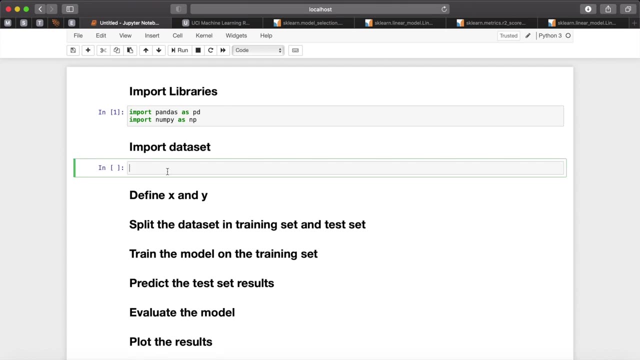 we will load these two libraries initially and we will import the other libraries as and when we need during the process of building our model. so we will Now. the next step for us would be to import the data set. Let's call it as data df, maybe, and let's read our data set that is in csv format. 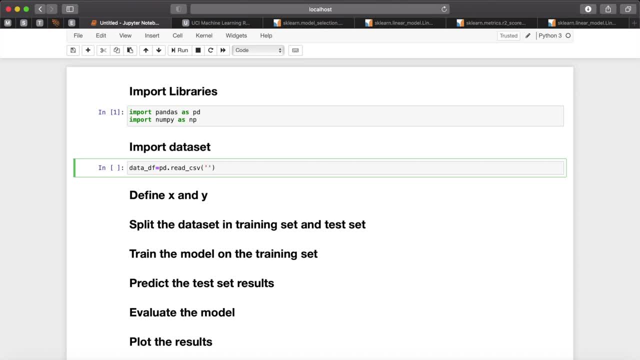 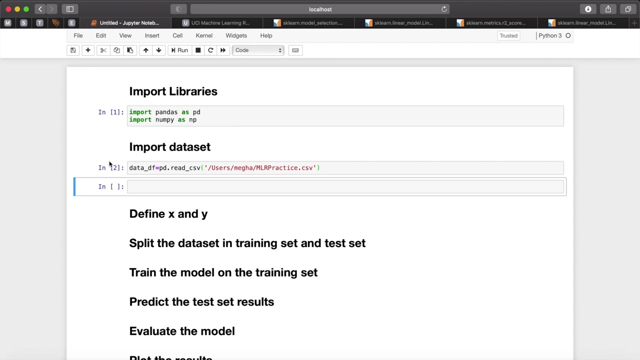 Let me just add the path of my file. You can add the path wherever you have stored your data set. Let me run it. Yes, Once our data set is imported and loaded, let's just check if it has been imported properly. So let me just add one more column and call the first five columns, first five rows of my data set. 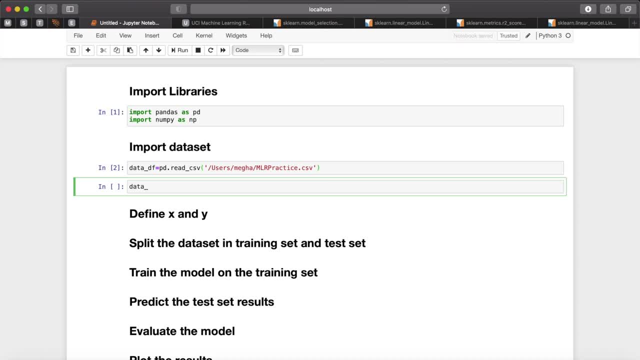 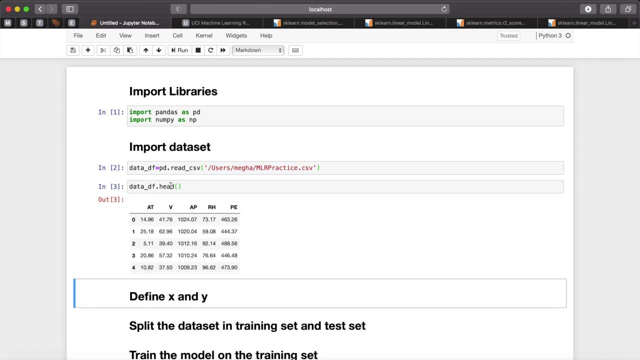 So to do that, I'll use dot head function. By default, it will display the top five rows of my data set, As we can see that the data is clearly represented and there is no error, which means that the data has been imported properly. 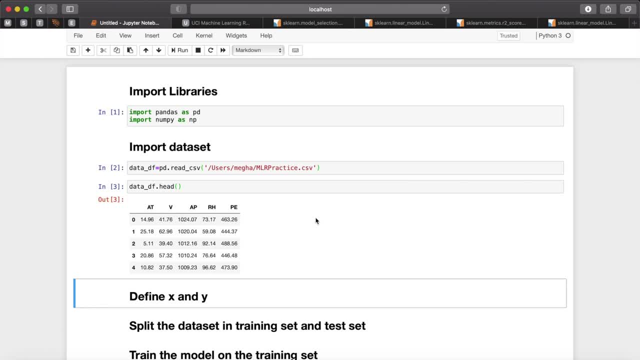 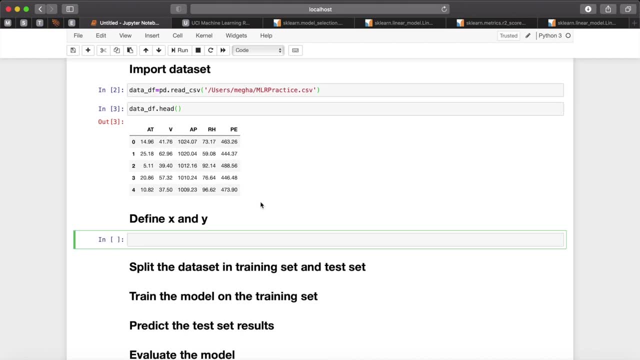 The next step for us would be to define our x and y, that is, our independent and our dependent variable. Let's first define our x variable, The code that we would use to get our data set. All the independent variables here, excluding the last column, would be the drop function. 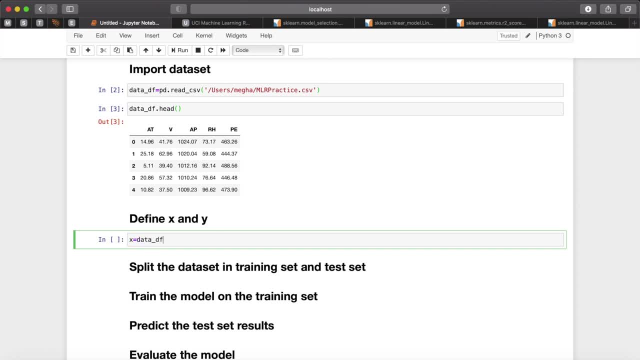 So that would be data set name: dot drop. The column that we need to drop is pe, So this pe And we need to drop the column. So x is equals to one And we need values in our x variable, So dot values. 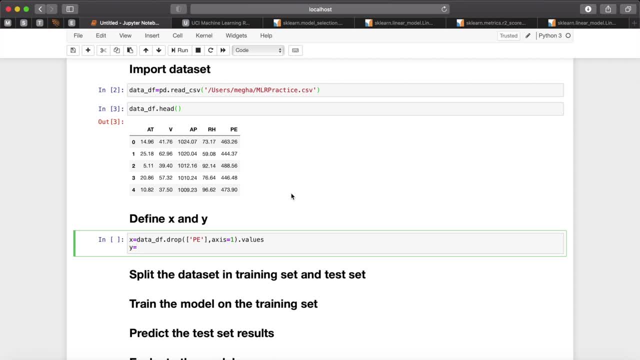 Similarly for y. Now in y we just need the last column, that is, p, which is our dependent variable. So for that we simply need to add And And ee In the data set, And That's it. 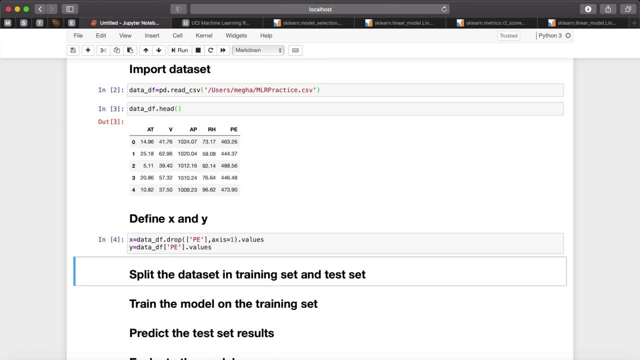 So once we run that There is no error which shows that our x and y are defined, Let's just check If all the values are properly added into x and y. to do that, Let's print x. so if we check, yes, for first four rows, the results are similar. again, let's just check. 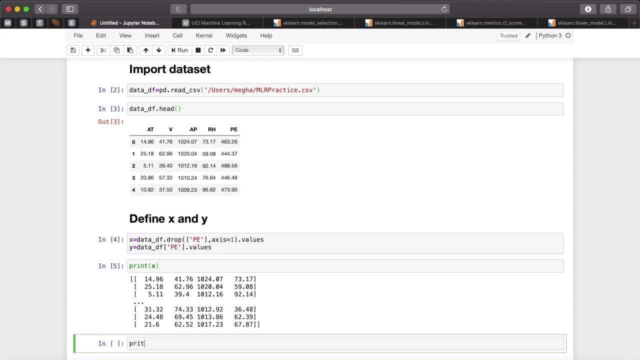 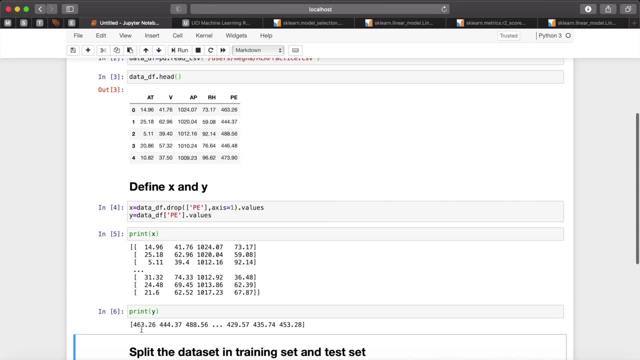 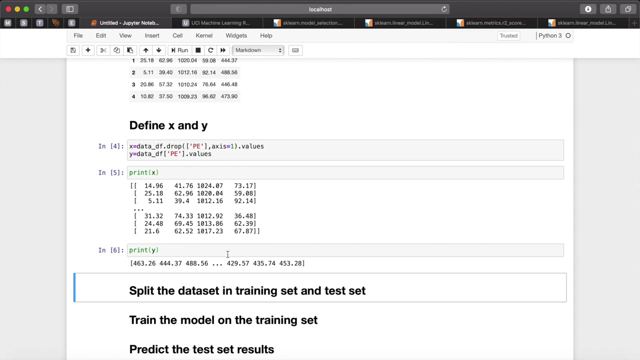 for y as well in the similar fashion, and this also shows the results. that shows that the values are properly added into y variable. once we define our x and y variable, that is, a dependent and independent variable- the next step that we need we should follow is split. 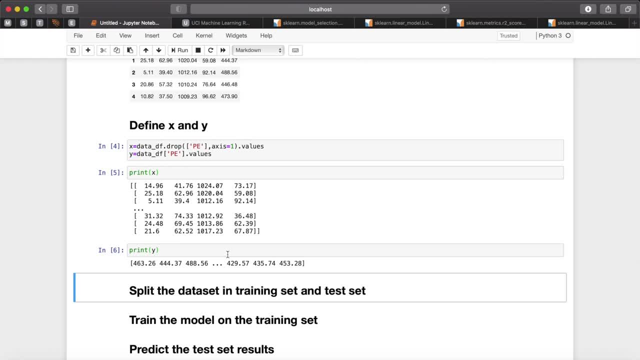 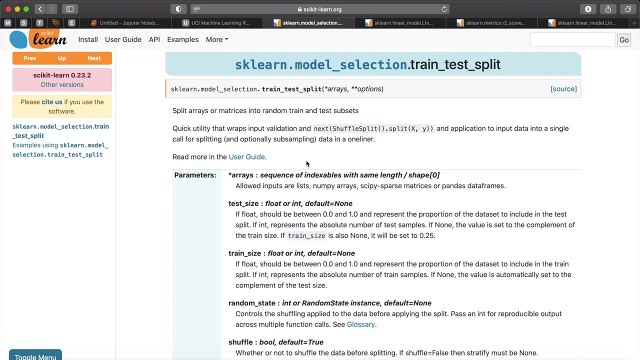 our data set into training and test set. in order to split the data into training and test set, we need to use the function from scikit library, so i have already added that here. so this is the train test split function that we are going to use from. 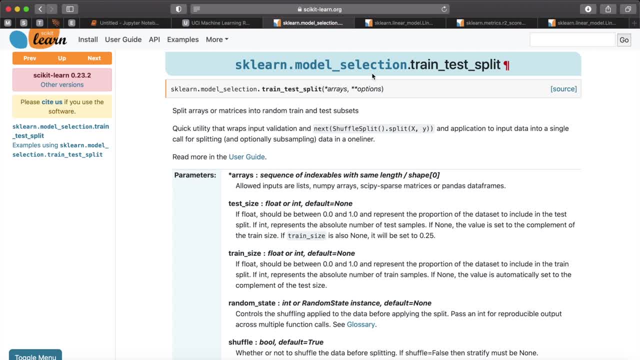 scikit learn. that is sklearn model selection. often, while building these models, we need to add different functions and we do not need to remember all these functions and their syntaxes. instead, we just need to know the kind of the library that we need and the model selection that we need to remember and the syntaxes that we need to remember and the 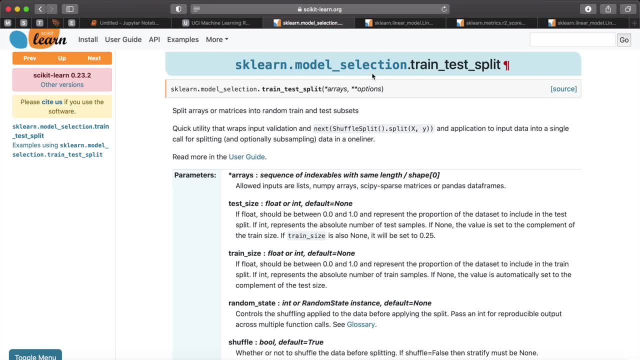 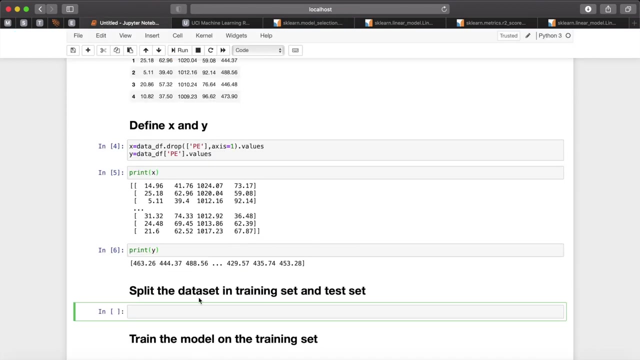 would be suitable for that particular model, and by accessing those libraries we can easily find the syntax for the function that we need to use. so here we are using train, test and split function from scikit library. so we'll just copy that here from scikit library, paste it here and 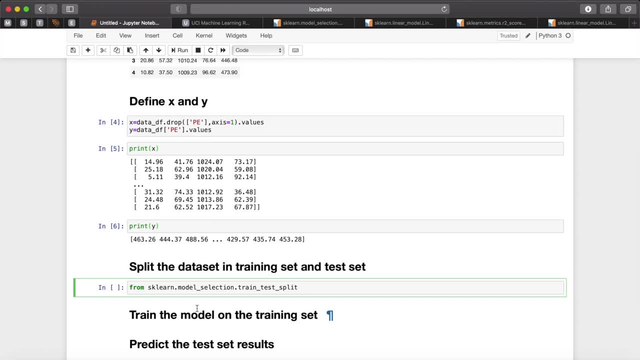 just make a few changes. which shows from model sklearnmodel selection we are importing train test split function. after we import that we need to put our x and y value variables into this train test split function. so to do that we will divide our data set into x train. 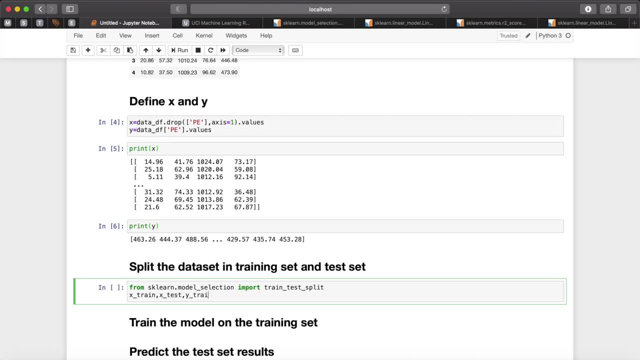 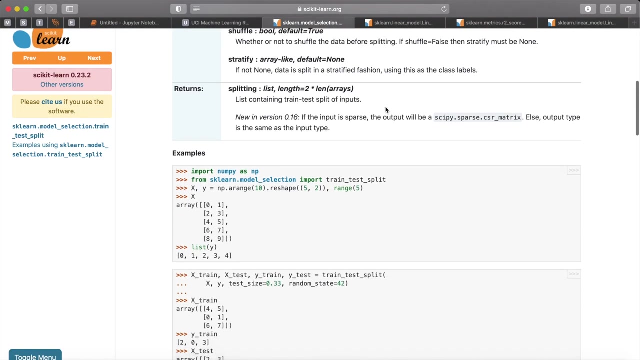 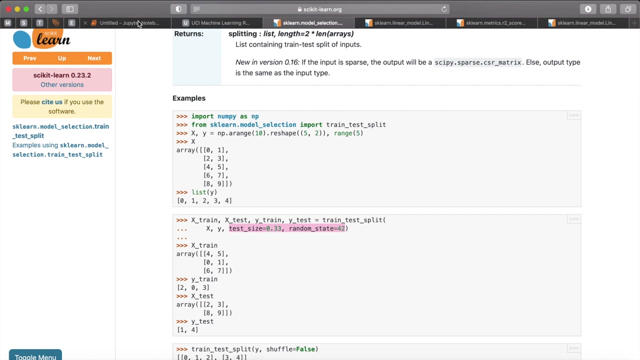 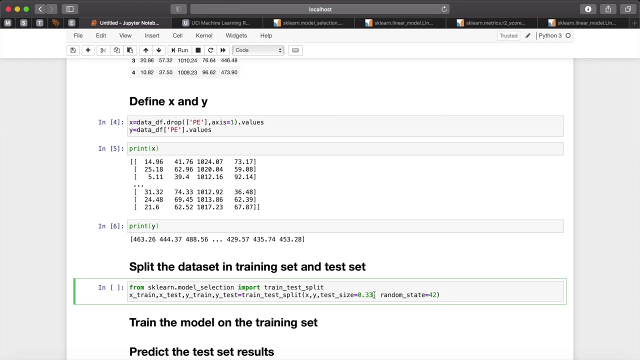 x test, Y train Y test from train test: split function of x and y. now once again we go to the model. we see that here we can define the test size and the state, random state. so test size would indicate how much percentage do we want to give to our training data set as well as test data set. 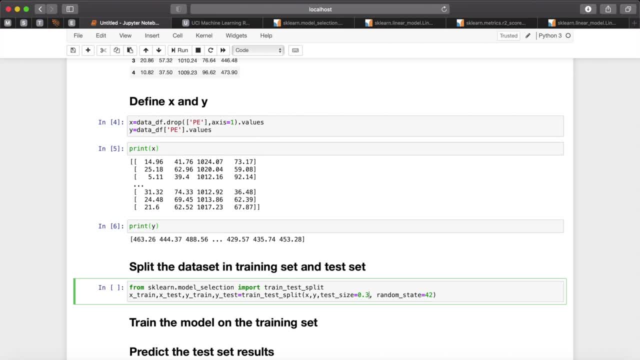 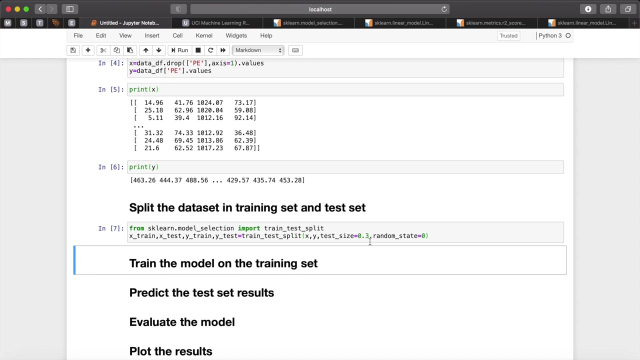 so here we will divide our data set into 70, 30, percentage and random state. let's keep it zero so that our results remain the same every time we run it. so let's just run it and see if there is no error. yes, so once we run it successfully, our data is. 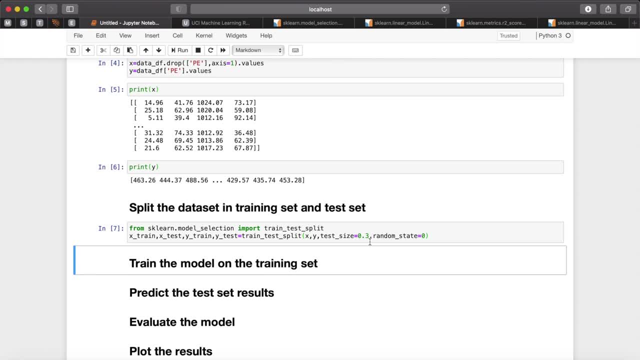 has been split into training set and test set. so after splitting the data set into training set and test set, the next step for us is to train the model on the training set. so for that we again then go to scikit library. first let me just add the cell here, and in the scikit library, 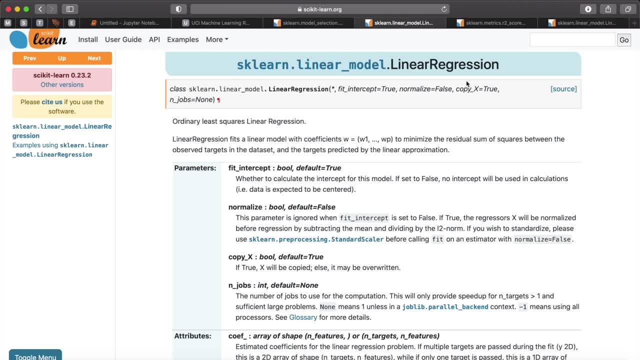 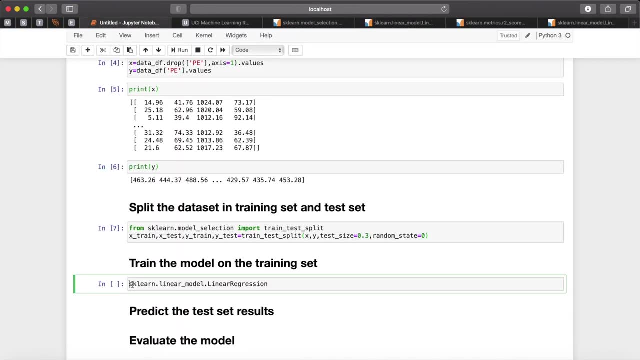 we will select linear regression function and from module sklearn linear model. again we will follow the same steps. from sklearn dot linear model, import linear regression, let's call the linear regression function and fit this model. again we will follow the same steps: from sklearn dot linear model, import linear regression, let's call the linear regression function and fit this model. 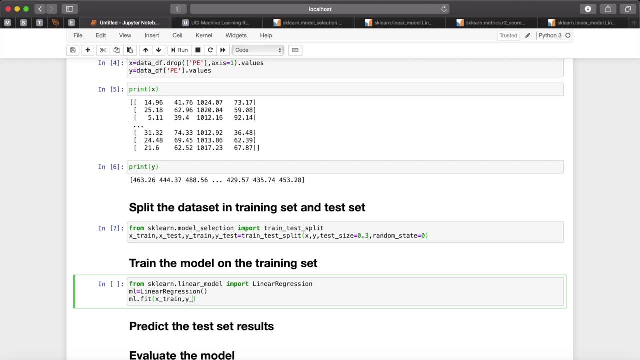 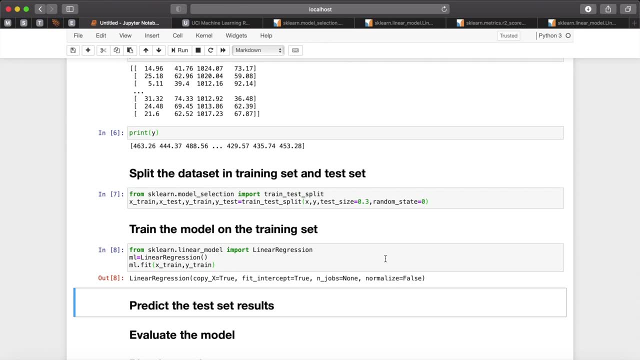 again, we will follow the same steps from sklearn dot linear model, import, linear regression. let's call the linear regression function and fit this model- x train and y train- into linear regression. After training the model on the training set, the next step for us would be to predict the test set results and see if we are getting. 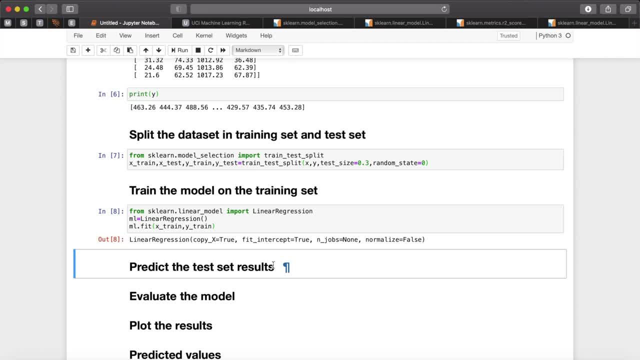 the accurate results. So to do that, we will call predict function and let us store it into y equals to m, l that we have defined here in our real linear regression function, predict function. And what do we want to predict? We want to predict from x test. Let us print the predicted. 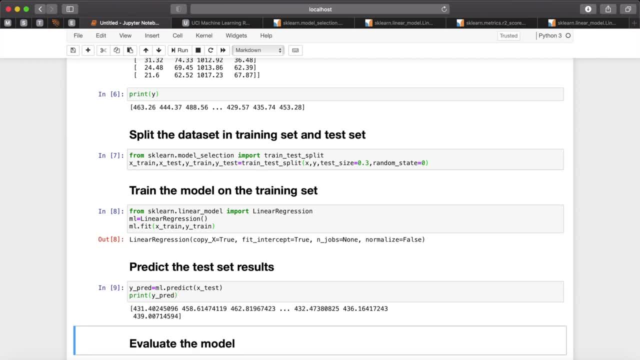 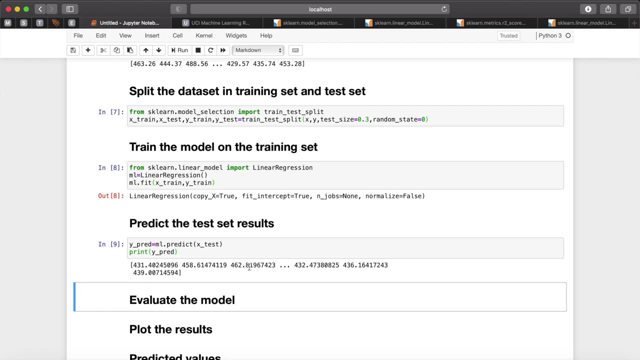 results. These are our predicted results, which here we can just see: the top four values and the bottom four values. In order to see it more clearly, let us take one more step And use the values of our x variable from the first rows of our data set and evaluate. 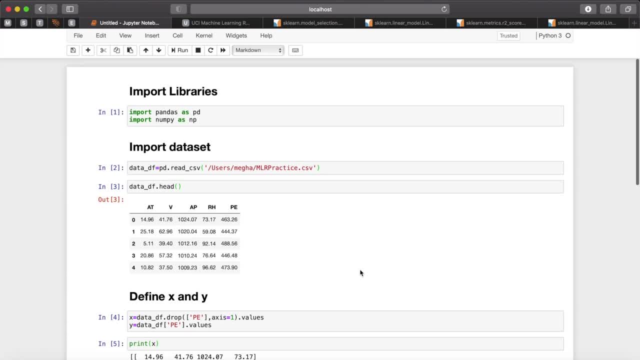 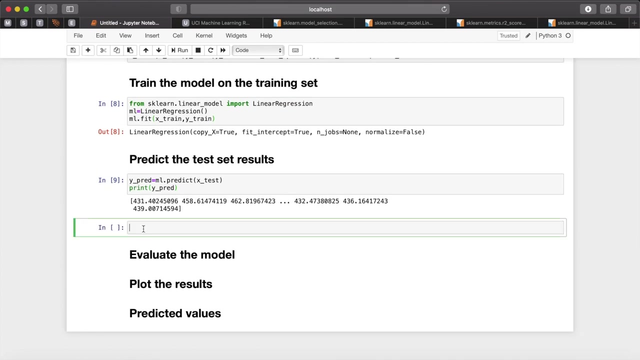 how close it is from the actual outcome, that is y. So we will copy the values of our first row and from four columns And let us just see what will be our results. m? l dot predict. You can add any other value here instead of the already existing value and you will get the predicted values of the 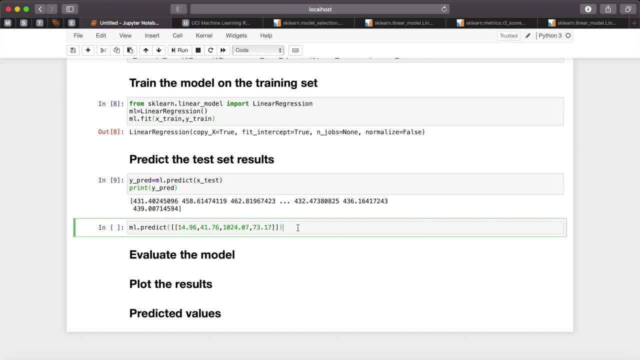 first row. So after we have copied the Timitte values from the text to the間 expression, we can see that we are getting the reflective values- the present members- that you input. So let us just check. So if we see the Y value, that is P E, here it is according to. 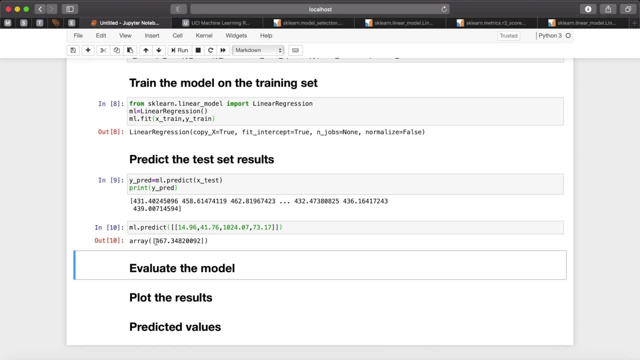 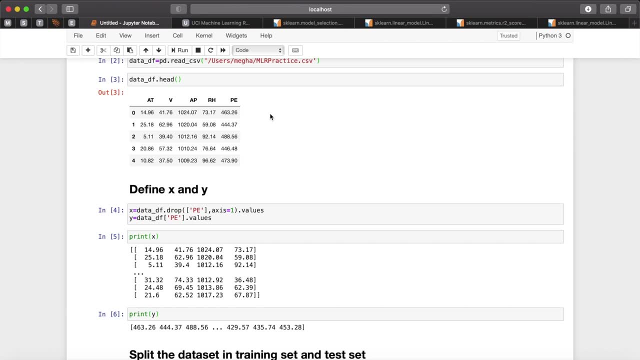 the model that we have prepared, the value of P E should be 467.3, 4.. Let us see the actual value, Which is this is 466.. Direction that I would say 463.36.. So it is close enough. I would not say that it is a comparison between the two. it should be pretty similar. So this is grinder Roger. There is their value and we will say for хоть the model that I know that it could be a terrific note. Okay, Let us see how much it will weigh the times. 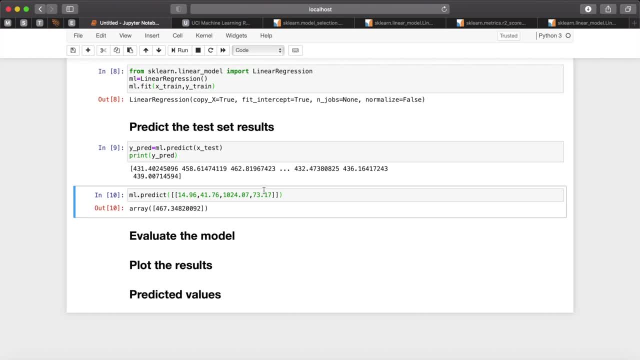 have been plotted. Now that we have predicted, it will be flowed out and this will be the completely accurate. however, it is very close to the actual value. now, in order to further evaluate whether how accurate our model is, how accurate our predicted values are, let us evaluate the model. 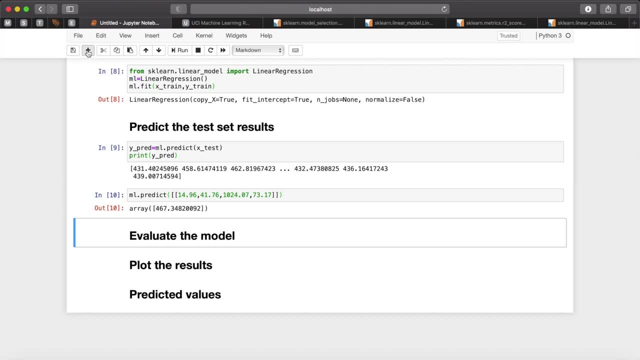 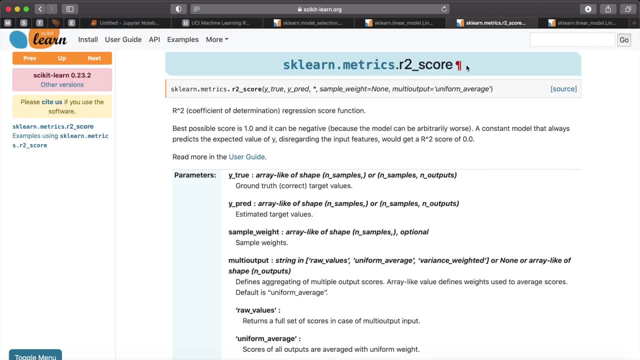 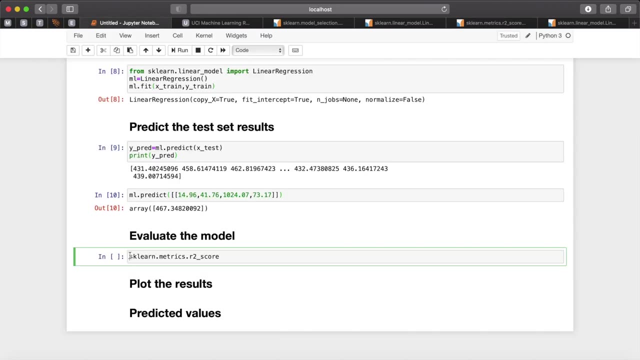 through r to score. so for that again we will go to sk scikit learn and here the function that we have is r to score and let's just copy it and from escalant dot matrix import r to score. the second step would be r to score of y test comma y. 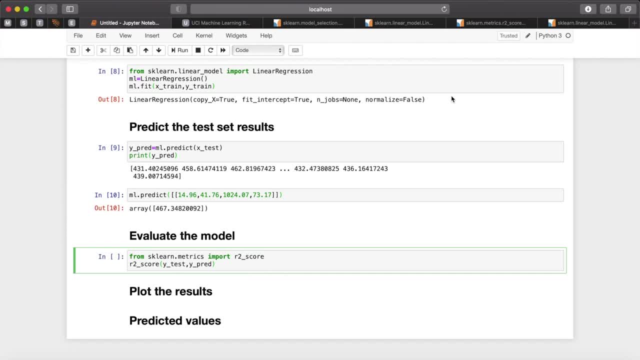 pred, because here if we see it says y true comma, y pred, so for us y true would be by test that we want the results for and predicted values. so here it shows that it is 93 percent. the score r to score is 93 percent, which is really a good score. so once we evaluate our model, 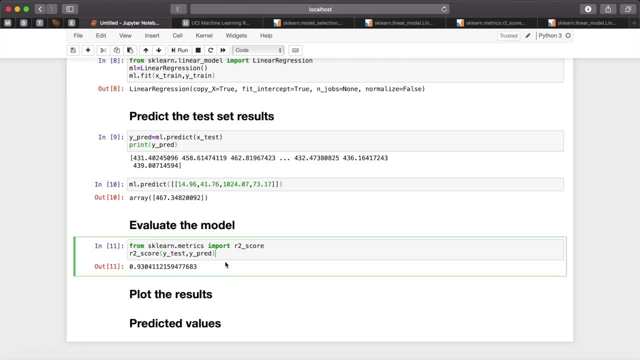 we already have our predicted values. we already have our, we have already evaluated our model. now the last step is to visualize the predicted results. so to visualize our predicted results, we will create a scatter plot. for that we would need import matplot libraries, plot dot pi, plot as pl. 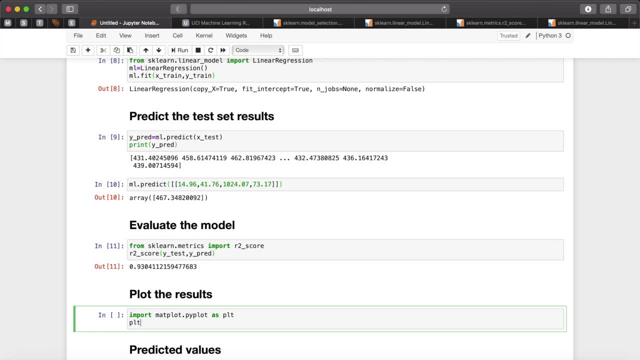 t. we will plot a scatter plot for by test actual versus predicted results. let's just change the size as well, otherwise it would be very small and may not be very the outcome may not be very clear. so figure size: let's keep it 1510 and X label is actual. 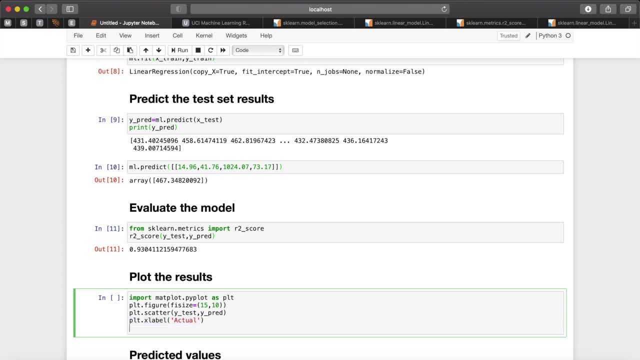 y label is actual variables for sign. saying x character is like the argument we just did the math x, but we can make someuded examples, for example, b to equal to 2 and so on, etc. focus here because we will be doing math and then we have an unclick, so using x global to analyze in reference to the future, like those we have to keep. x and so by sometimes update once every couple come to the actual number, shape changes sometimes some sei to u5noset platform in the description of thevor vkn reconstruction College of Mathematics. we also have most of you that we would want it, but I don't want to clear those biggerれ. 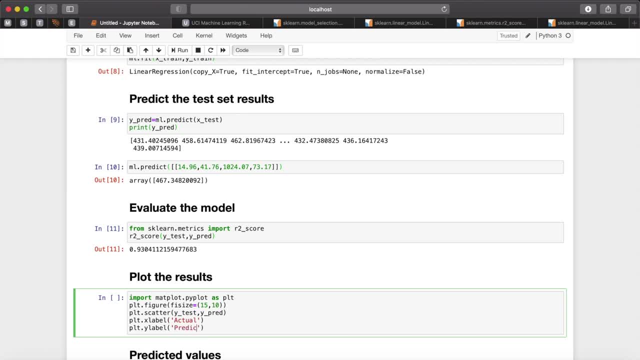 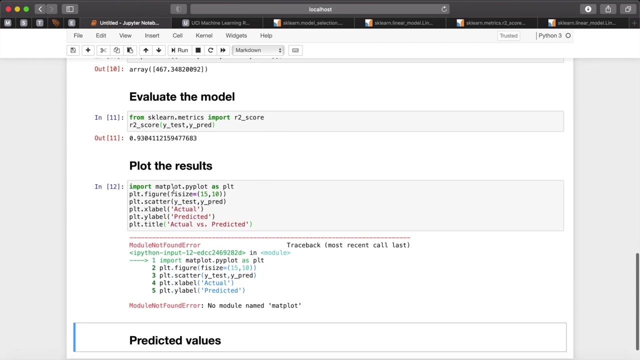 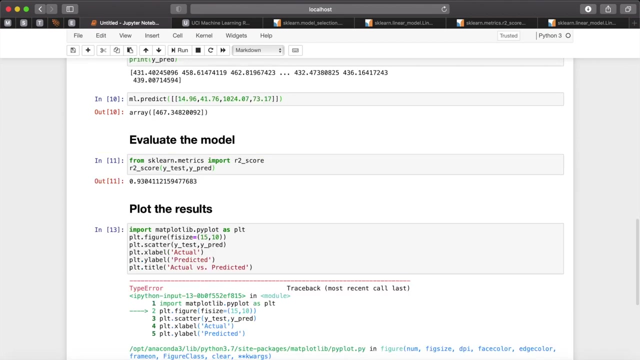 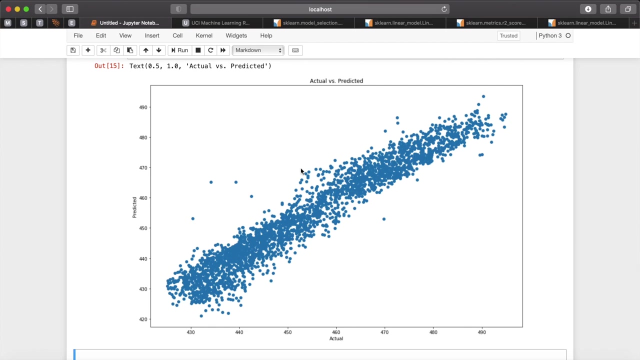 would be predicted and the title is actual versus predicted. let us see what our results are. we have got an error import matplotlib. sorry about that. yeah, so when we see the results and compare our actual versus predicted values, we see that they are pretty close enough. there are only a few exceptions here and there. however, if we in 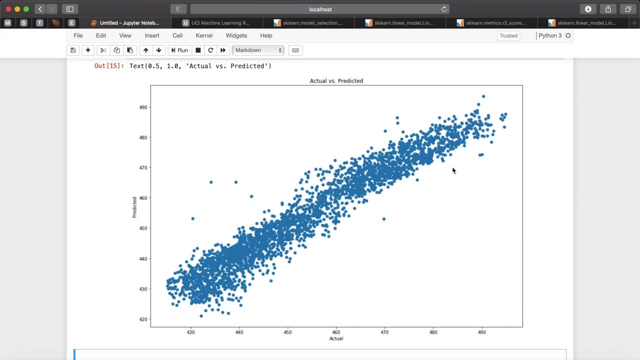 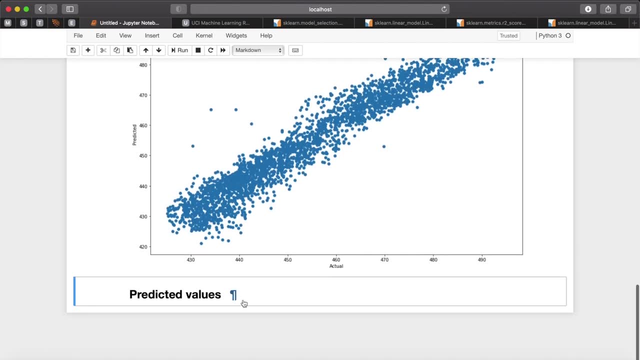 a. however, if we look at our model, this this gives a pretty good predicted values. so let's just go ahead and print the predicted values of our model. to do that. let's add, put the values in a data frame and let us do one more comparison while we are adding these values. actual value would 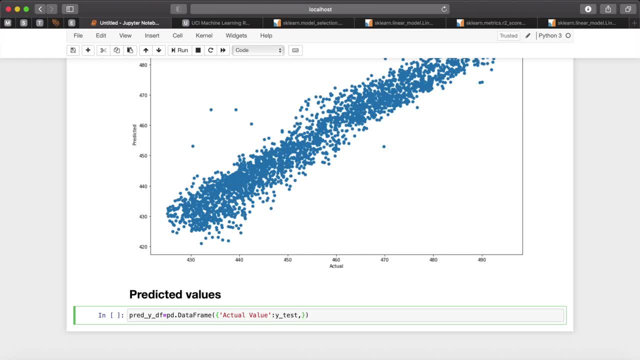 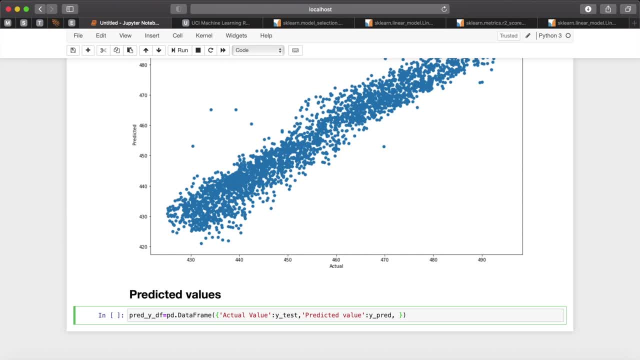 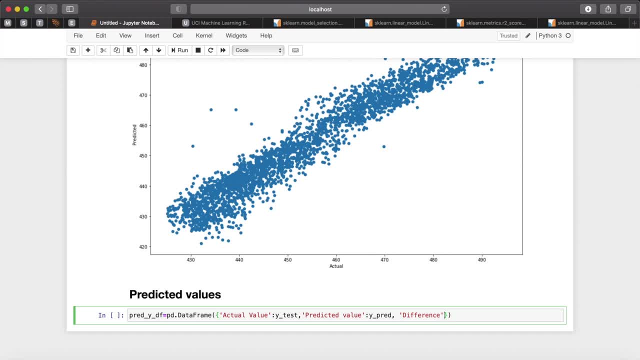 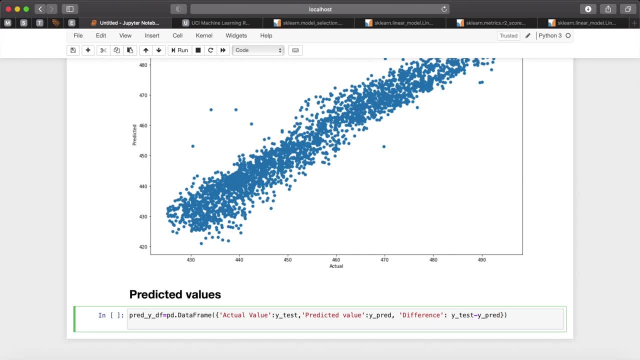 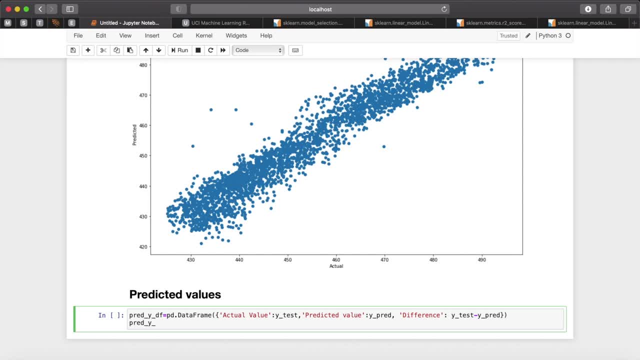 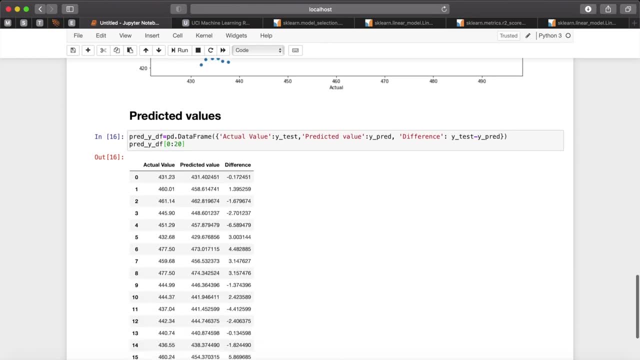 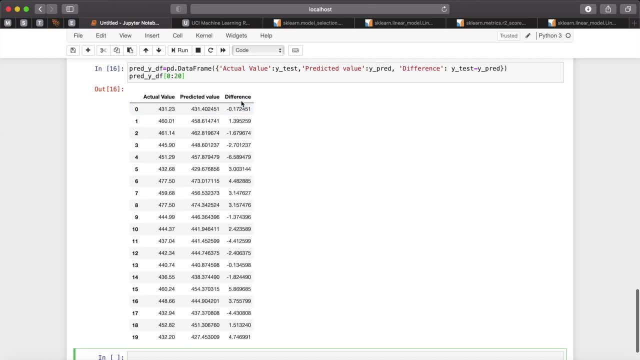 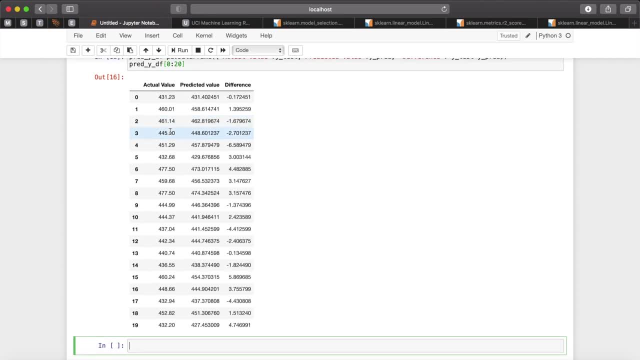 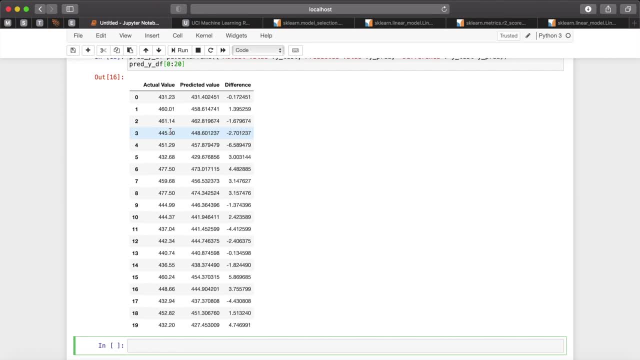 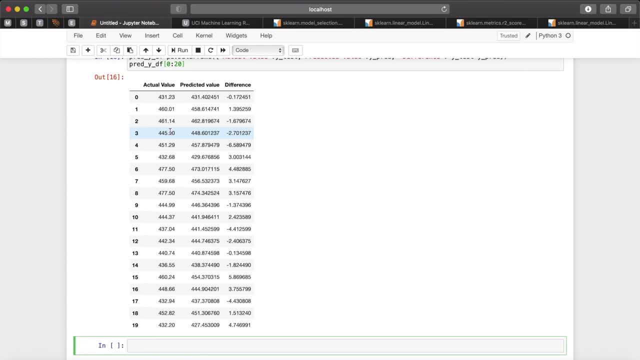 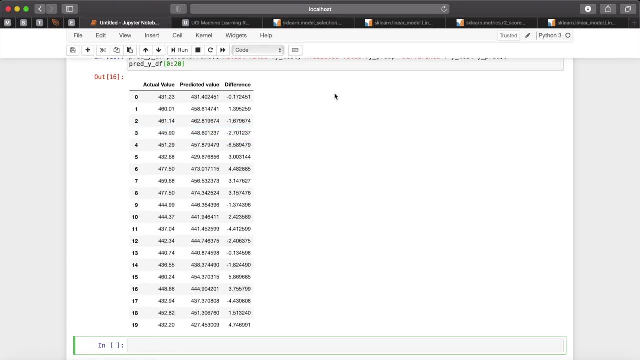